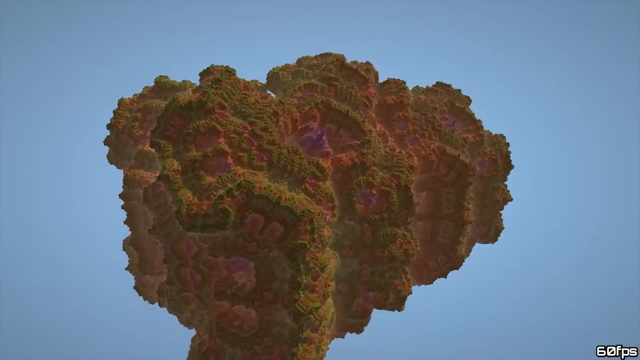 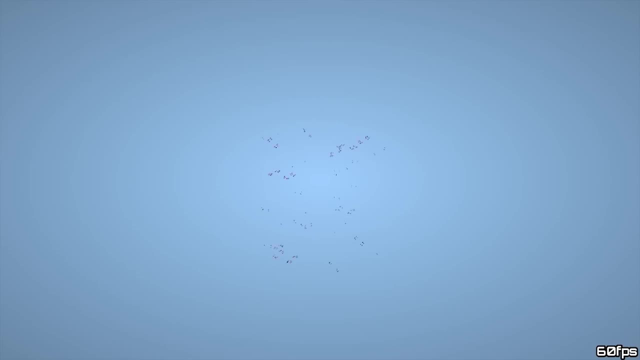 Yeah, 3D fractals are awesome, but then why do you rarely see procedural rendering used in games? I mean, ray marching unlimited objects in real time seems really useful, right. Well, the problem. is sure, there's efficient ways to draw these objects, but how do you actually? 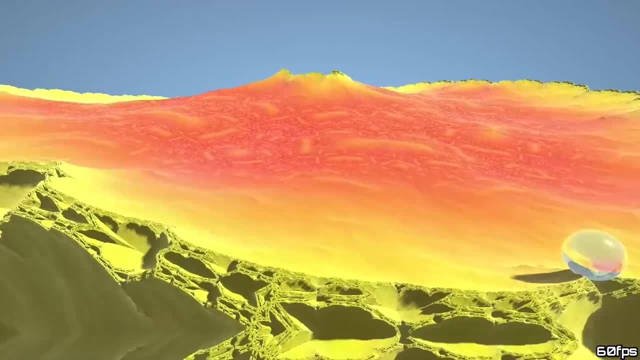 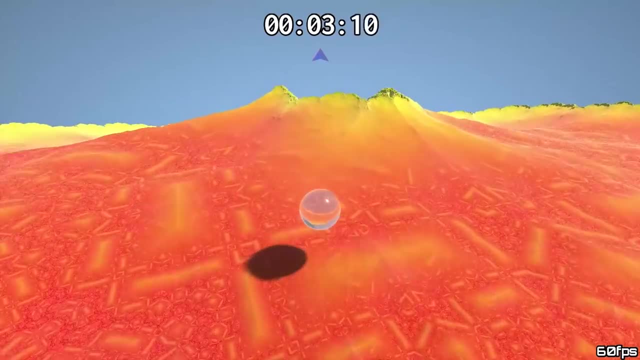 interact with them. Well, I'm going to show you Marble Marcher. It's a proof of concept to show that fractals aren't just fun to look at, but real games can be built with them using a fractal physics engine. The download link and source code are in the description. 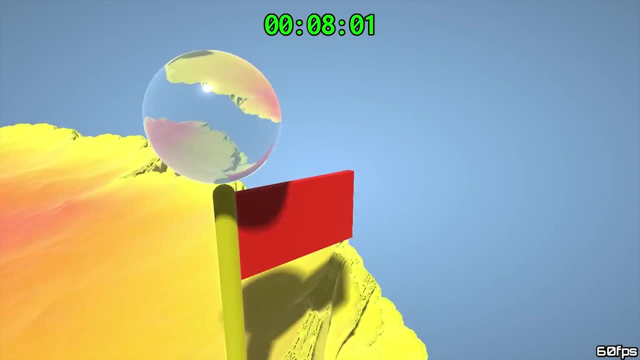 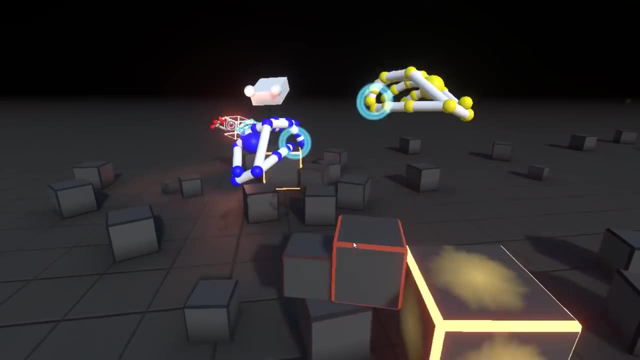 If you want to understand how ray marching works, you'll definitely want to check out my other video on that first. otherwise some of this video might not make any sense. So what do we actually need for a physics engine? The most critical and difficult piece. 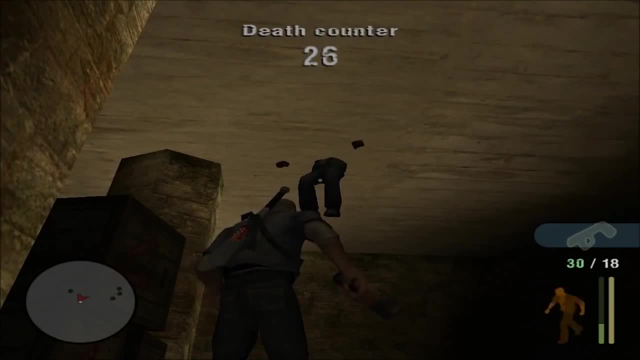 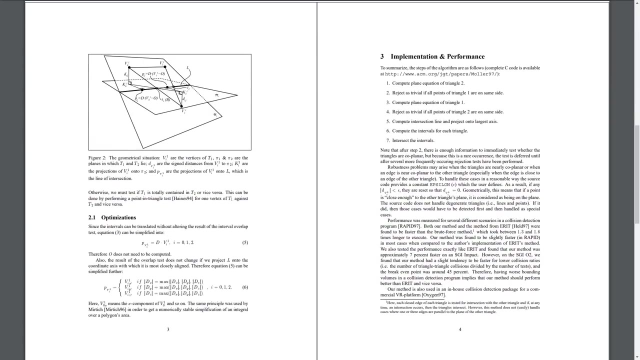 is collision detection, and that's why it's often the biggest source of glitches in modern games. Collisions are fundamentally difficult because the math is complicated and expensive, so games make a lot of approximations and they're always trying to balance accuracy. 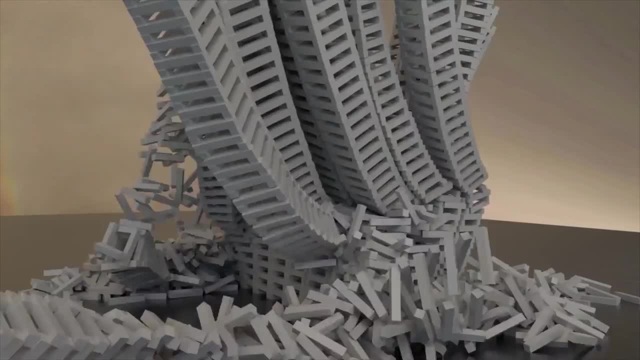 with speed, And even then, after a few thousand objects, things typically start to slow down. So what do we actually need for a physics engine? Well, the most critical and difficult piece is collision detection. Now we should have an opportunity to do better, because 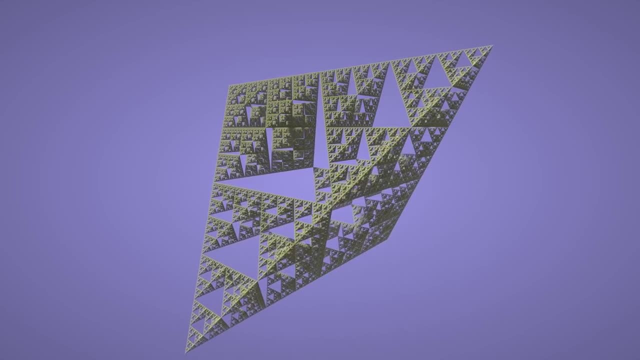 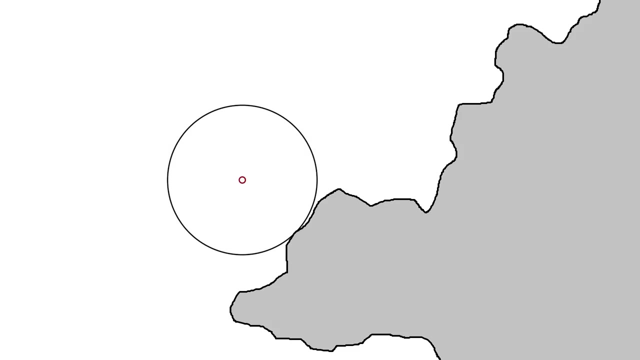 rendering a fractal is really only rendering a single root object, with a bunch of transformations and folds applied to it. So how can we transfer this to the physics? Remember how fractals have a really efficient distance estimator. Well, this is actually really useful If our 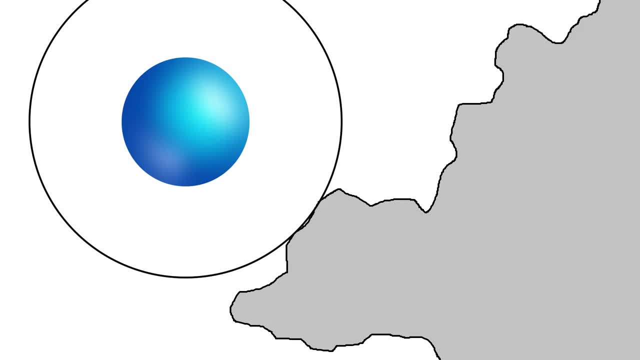 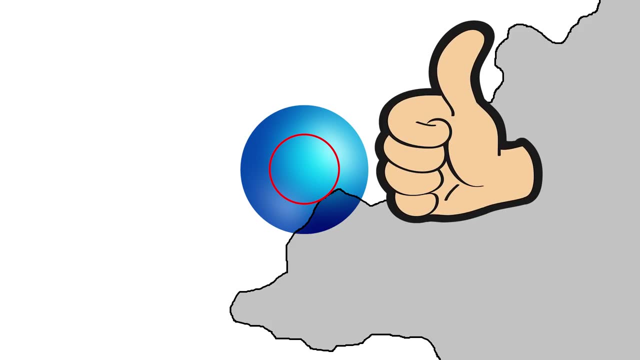 object is a sphere with a radius, then just by checking the distance estimator we can immediately know if we're intersecting or colliding with the fractal if the distance is less than the radius. So problem solved right. Knowing that you're colliding with something isn't enough, because you also have to know. 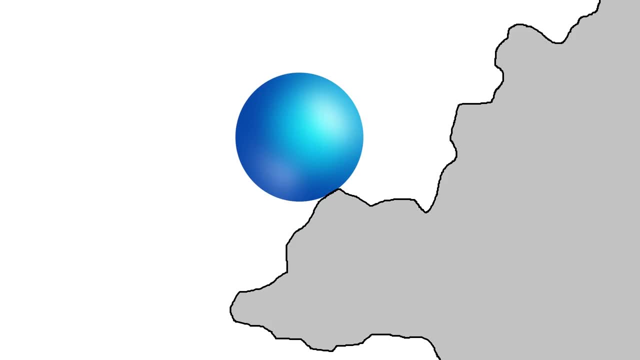 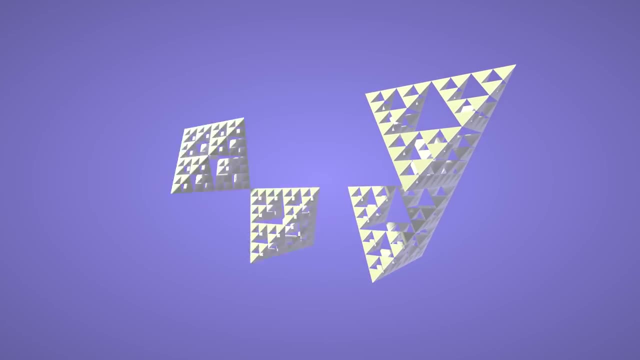 how to react to the collision and un-intersect yourself, And it's not obvious how we would get that information efficiently. So I'm going to put a big twist on everything. Normally, you compute folds and transformations a bunch of times and then finally take the distance. 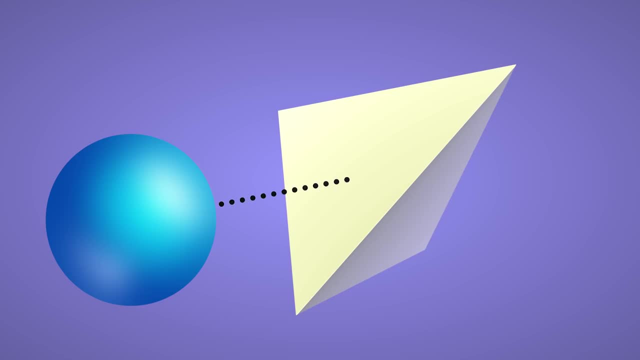 estimate of a root object. But let's say: instead of computing the distance, you compute the closest point. Okay, but the closest point on the root object isn't actually that useful. Once we have it, though, we can just un-intersect the object. So let's say, instead of computing,